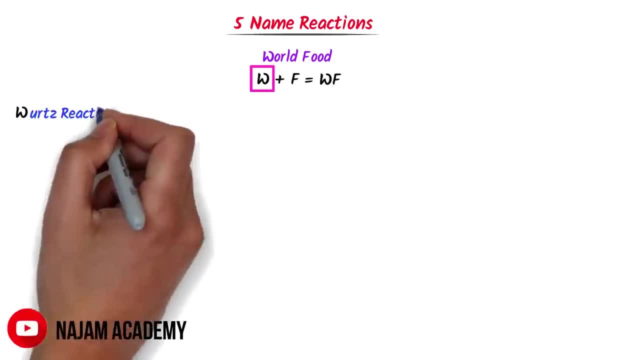 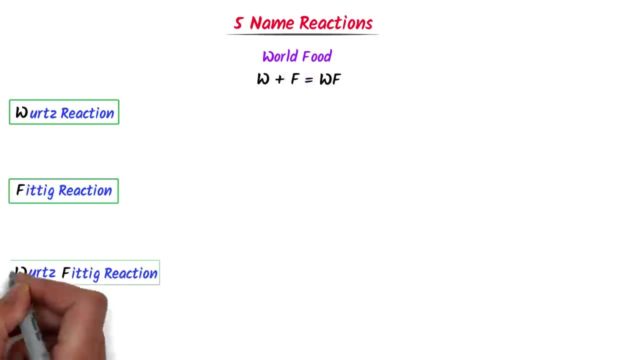 Now listen carefully. This W stands for words reaction, This F stands for fatigue reaction And this WF stands for words fatigue reaction. Now think about a very unique girl in your school or college. Let her name is Rukhsana Bukhsana. She loves to eat dried eggs. Remember that I. 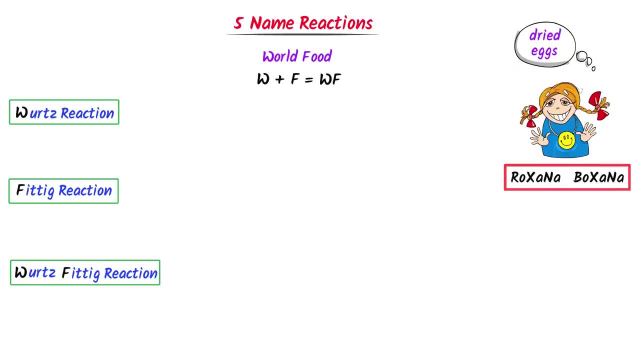 capitalize every second letter of Rukhsana Bukhsana. Now, in case of words reaction, I take R and X. It is alkyl halide. Note it down that here X is halogen like chlorine bromide. Now I take R and X: It is alkyl halide. Note it down that here X is halogen like chlorine. 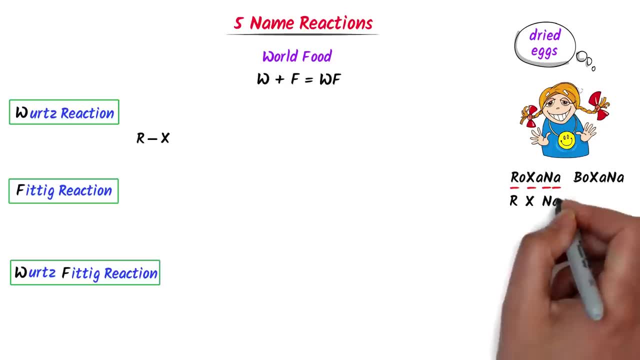 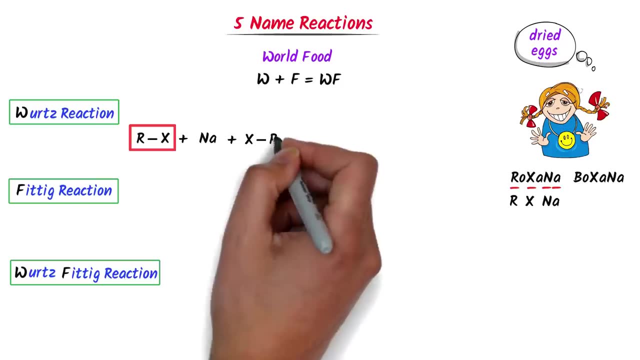 bromide for photosynthesis, alkyl road blood for blood, fluorhidrate for plant production, ammonium bromide for food with citric acid for carbon устрой race lime verschiedine, hesidic argon. for scholars add it. 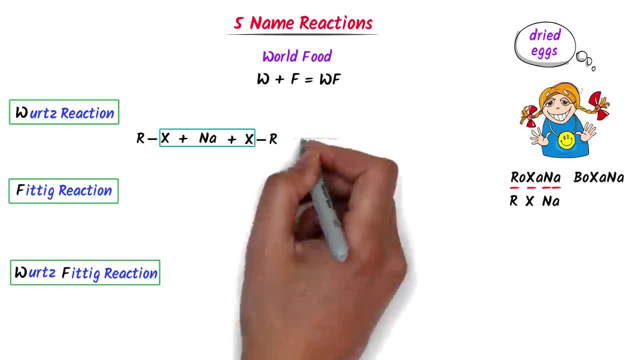 valium hydrochloric acid. iv butane for skeletons with barb. valium ribosomesmachium. This R and this R will combine together to form alkane. This dried X stands for dry ether. Thus this is the Wurz reaction. 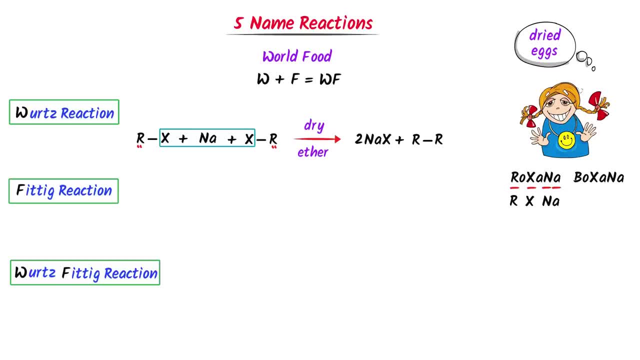 Now, in case of fatigue reaction, I consider Buxana, This B, and Buxana stands for benzene ring, And this X, or halogen, is attached to it, Plus this N-S stands for sodium, Plus I take this benzene and X. 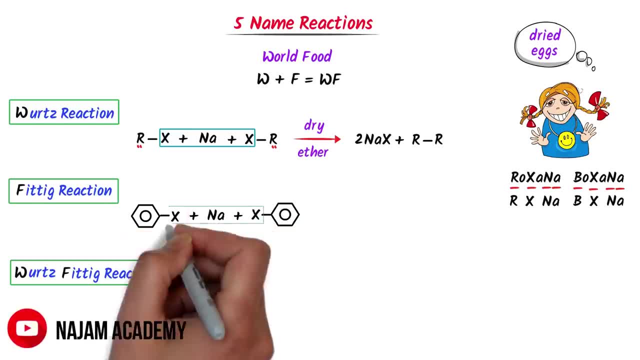 I rewrite it here Now. sodium will react with these two halogen to form 2-sodium, halide Plus. this benzene and this benzene ring join together to form diphenyl. This dried X stands for dry ether. Thus this is the fatigue reaction. 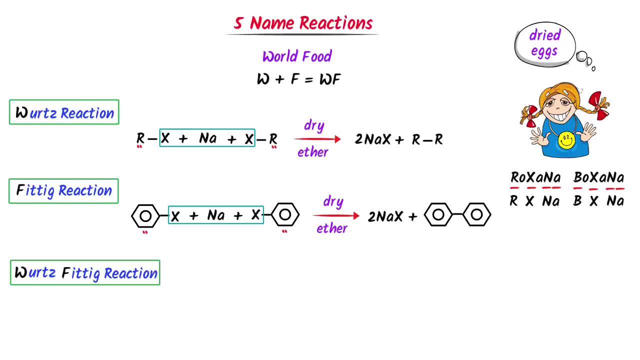 Thirdly, in case of Wurz fatigue reaction, I write sodium. I take the first reactant from Wurz reaction and first reactants from fatigue reaction. We know that sodium will react with these two halogen. I take 2-sodium halide. this benzene ring and this alkyl join together to form alkylbenzene. 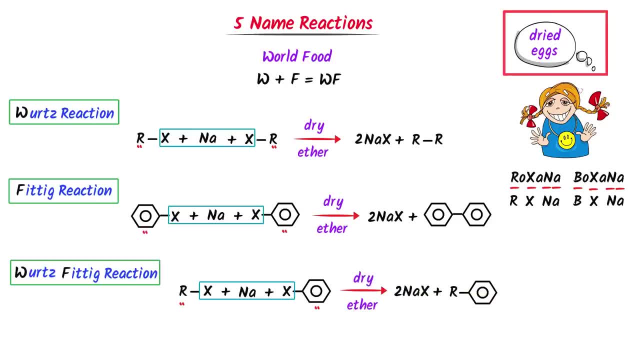 This dried X stands for dry ether. Thus this is the Wurz fatigue reaction. Thus, using this trick, we can easily learn these three reactions. Fourthly, this F also stands for Finkelstein reaction. Now let's consider the sister of F. 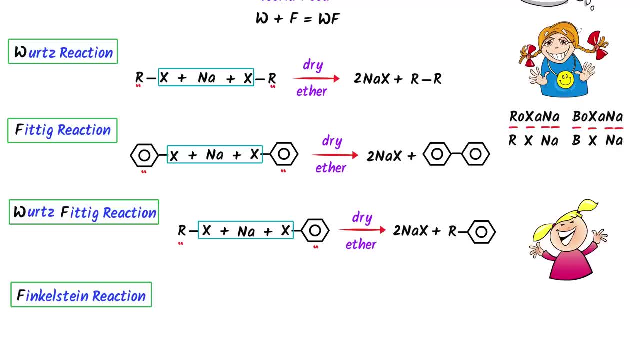 Now let's consider the sister of F. Let the name of her sister is Rukhsana India. She loves to eat dry apple. Remember that I again capitalize every second letter in the Rukhsana India. Now, as usual, I take R and X. 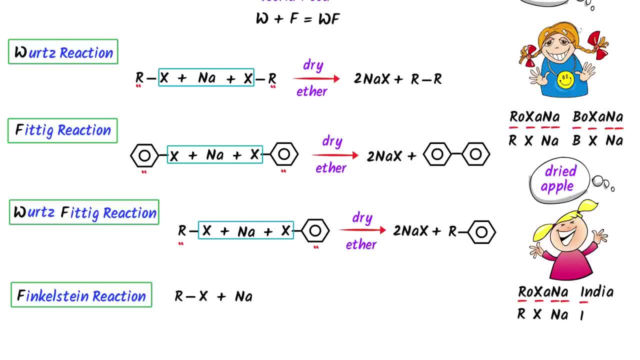 Then I take sodium. This I in India stands for iodine I. We know that metal like sodium loves to react with this halogen, So we get sodium halide Plus alkyl iodide. This dry apples mean dry acetone. 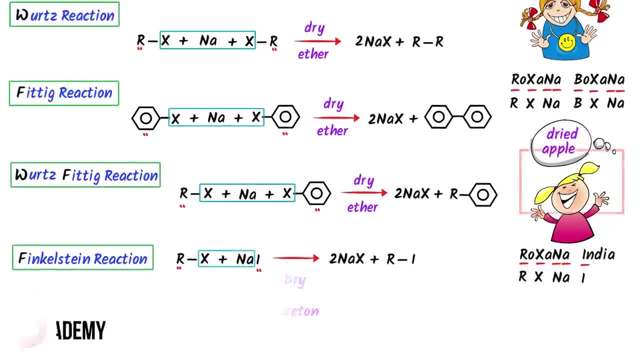 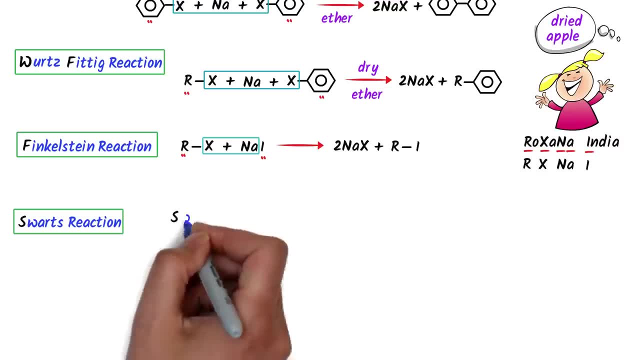 So this is the complete reaction of Finkelstein reaction. Fifthly, consider Swart's reaction. Remember that in the Swart I select S-A-R. Now this S-A-R reminds me Swizerland flag This R and Swizerland remind me R-X. 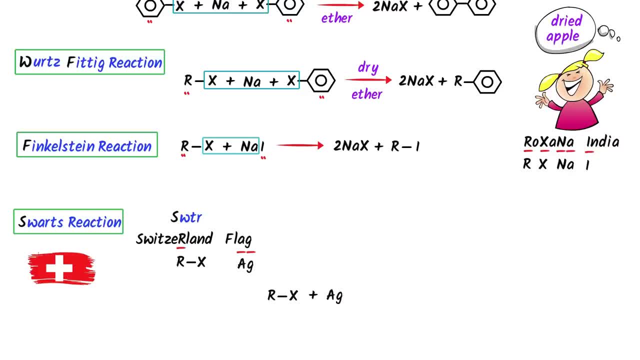 Now the A-G, and the flag reminds me S-A-R, Now the A-G, and the flag reminds me S-A-R- Now the A-G, and the flag reminds me A-G-R-SILVER, Now the A-G, and the flag reminds me S-A-R. 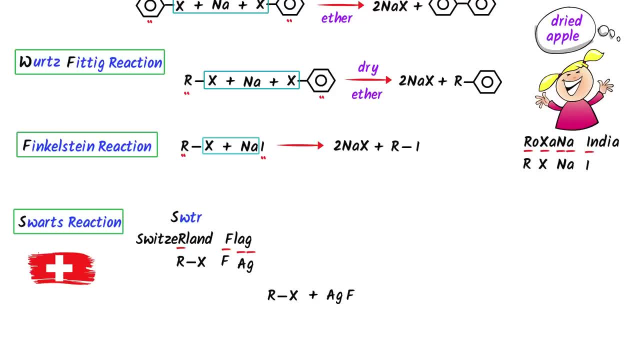 F, and the flag reminds me F-Fluorine. We know that metal like silver reacts with halogen X to form silver halide, While this fluorine and alkyl combine together to form alkyl fluoride. So this is the Swart's reaction. 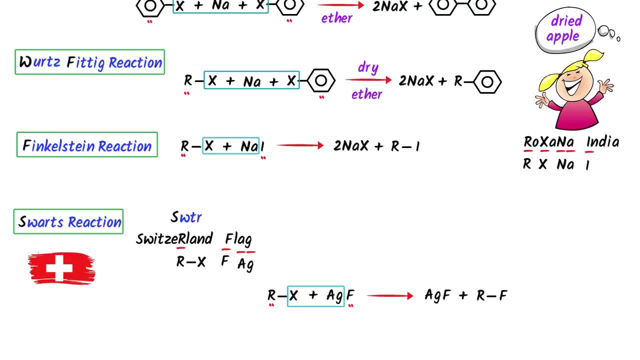 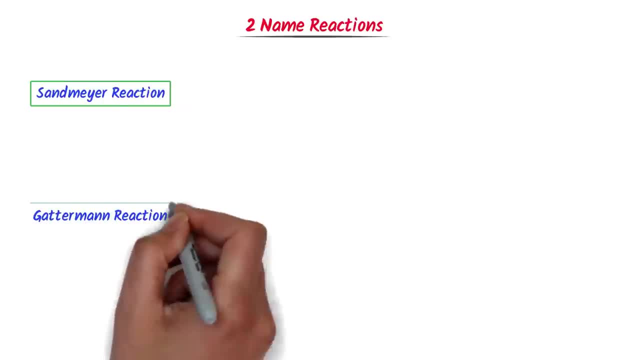 Thus noted down this: five reactions which are somehow connected. Now let me teach you two more reactions like Like, Send me reactions and getterman reaction. Now in sand mirror there is word mirror. We know that mirror controls a specific area like a town, bazaar, etc. Let here the mirror is Mr Najam, So I say Najam. closed. 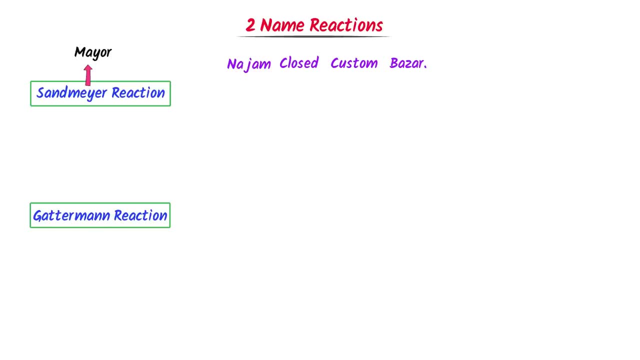 custom bazaar. Let me repeat it: Najam, closed custom bazaar. This close reminds me closed structure of benzene. This N Najam stands for nitrogen gas N2.. Remember that I need to put halogen after every element. This CL and close stands for chlorine. Now this CU and custom. 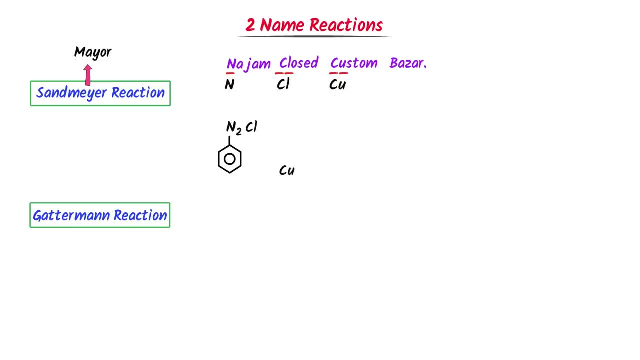 stands for copper. I again need to put one halogen like chlorine- This BR. and bazaar stands for bromine. We know that BR does not exist independently. I put hydrogen with it, So these are the reactants of this reaction. Now we can easily guess its products. I cut hydrogen. 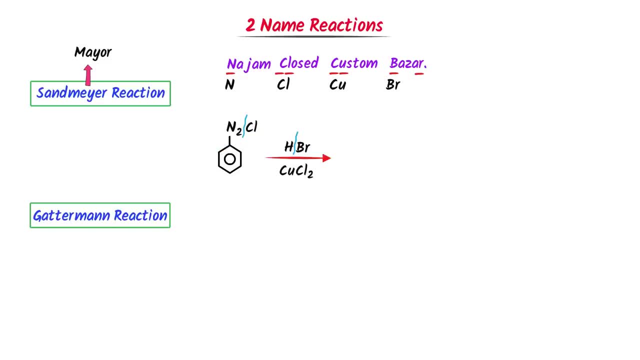 and bromine. I cut nitrogen and chlorine. This nitrogen gas will evolve as nitrogen gas. This chlorine and H combine to form HCL. This benzene ring and bromine react together to form alkyl halide. So this is the sand mirror reaction. What about getterman reaction? Well, 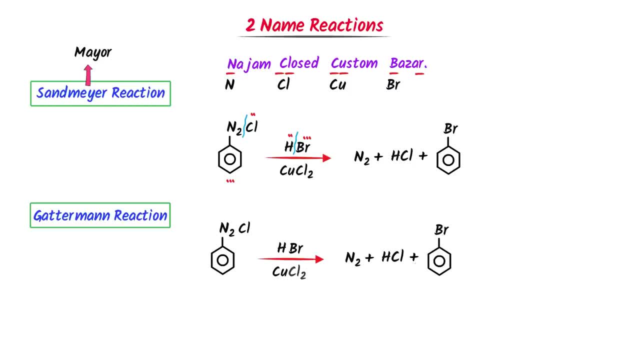 I rewrite the sand mirror reaction. Now listen carefully. I cut only copper chloride and replace it with copper powder. Let me repeat it: I cut only copper chloride and replace it with copper powder. I get getterman reaction. So this is the getterman reaction, Let's note. 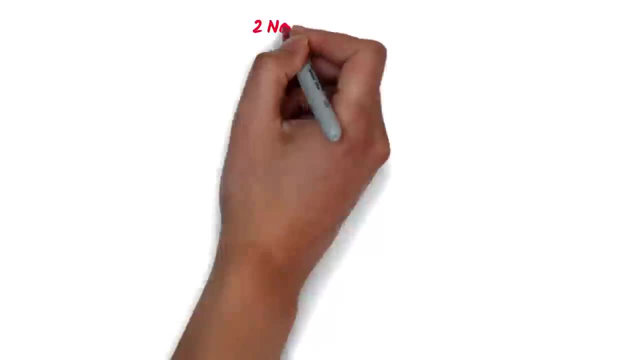 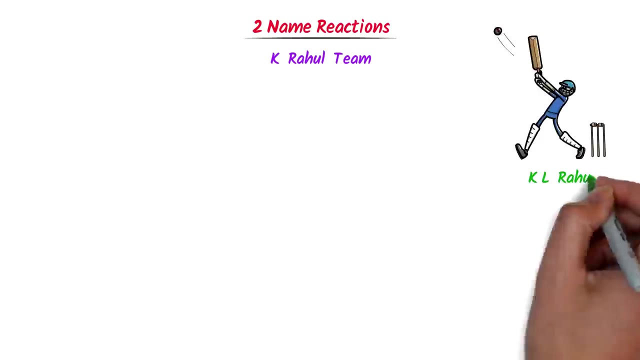 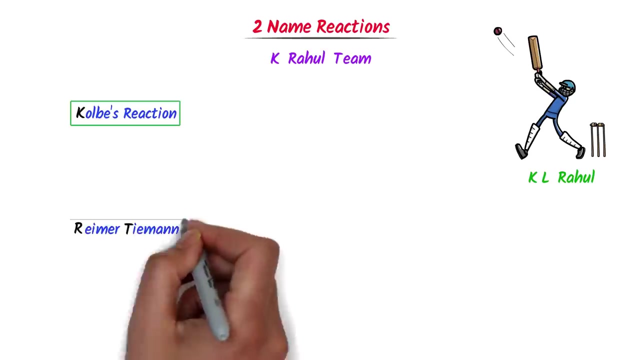 it down. these two reactions. Now I will teach you two more reactions. I write K Rahul team. Remember the famous cricketer K L Rahul Here? this K stands for Colby's reaction and this R and T stands for Rimmer-Thiemann's reaction. Now listen. 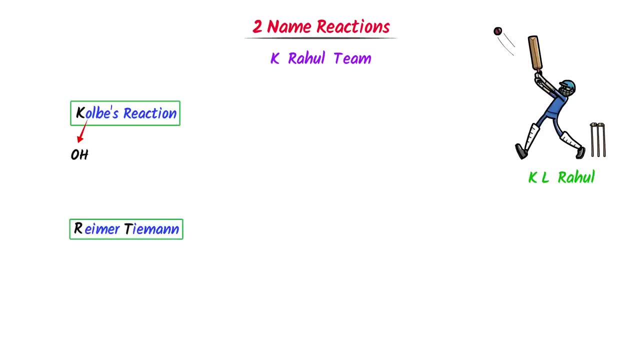 carefully. This O and Colby stands for OH and carbon dioxide. This B stands for benzene and base plus salt. Thus I take this OH and I attach it to benzene ring, I get phenol. Secondly, I write carbon dioxide, The base is sodium hydroxide and 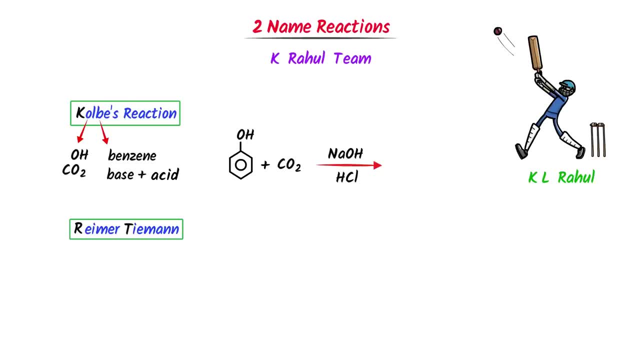 the acid is HCl. These are the reactions of this reaction and we can easily guess its products. I take this phenyl and I write it here Now. I select this carbon dioxide and H of base. Lastly, I attach COOH to this benzene ring. 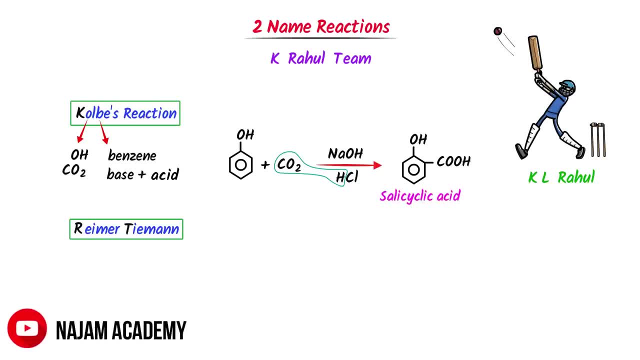 I select this carbon dioxide and H of base. Lastly, I attach COOH to this benzene ring. I get salicylic acid. So this is the Colby's reaction. In case of Rimmer-Thiemann's reaction, I rewrite the above reaction. Now listen carefully. I cut this O2 and 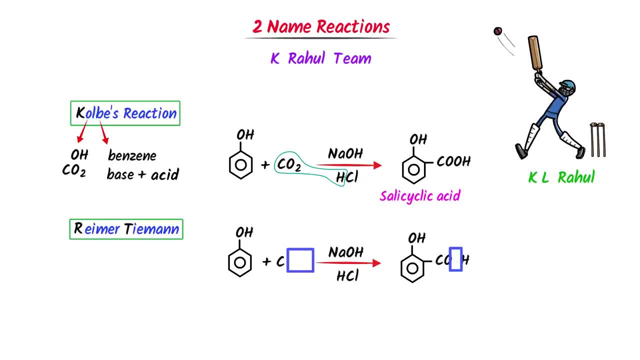 this oxygen of COOH. I replace only the O2 by Cl3.. Let me repeat it: I cut this O2 and this O of COOH. I replace only this O2 by Cl3.. We get a new substance and we call it salicylaldehyde. Thus, this is the Rimmer-Thiemann's. 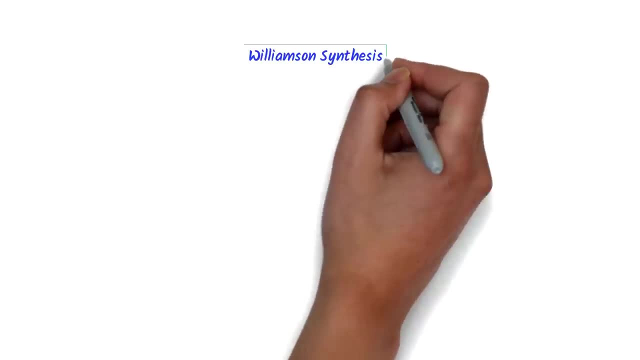 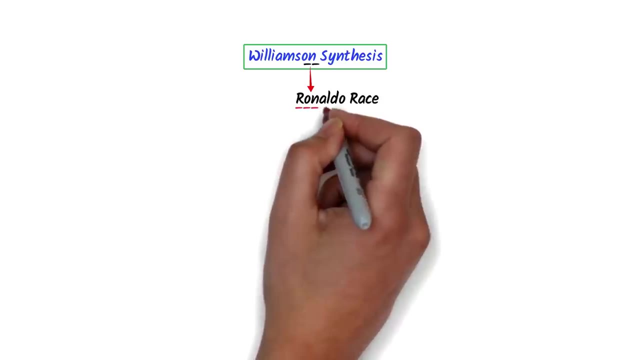 reaction. Now let me teach you Williamson synthesis. This ON. and Williamson reminds me Ronaldo Reyes. This RONA is sodium alkoxide, This R and Reyes stands for RX, alkyl halide. These are the reactants of this reaction. Sodium being positive will attack on halogen. We get sodium halide. This RO and this R combine. 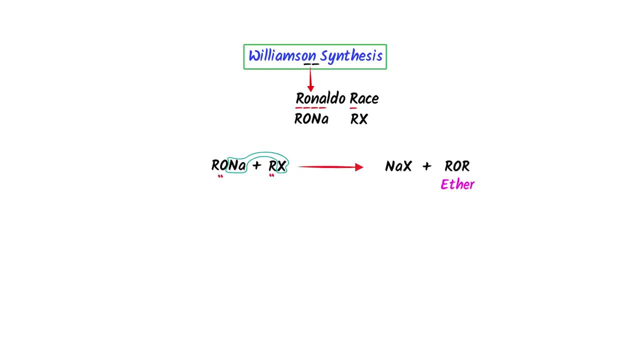 together to form ether. So this is the Williamson synthesis reaction. Now let me teach you, Stefan, reduction reaction. Well, I select R C and N in reduction. Now this R C and N stands for alkyl cyanide. Now, these are the three letters, as you can see in the video. Now I 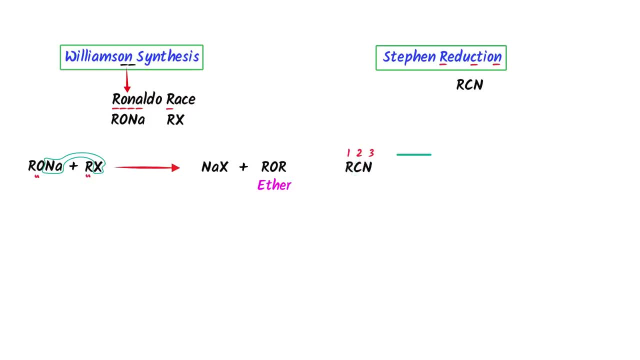 write here three dashes. Now I select S and N and Stefan. It stands for SNCl2 or Tünk chloride. This dash is for acid like HCl. This dash is for water. These are the reactants of this reaction. I replace this nitrogen by HO of water. I write R, C and HO. This is LD High. oxygen. Let me change this nitrogen by HO of water. I write R, C and HO. This is LD: High oxygen. Let me replace this nitrogen by HO of water. I write R C and HO of water. This is LD: High oxygen. 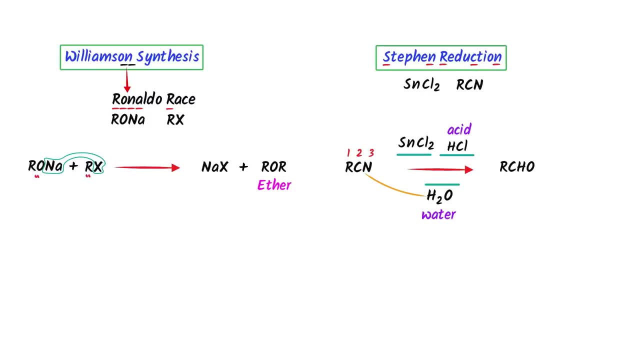 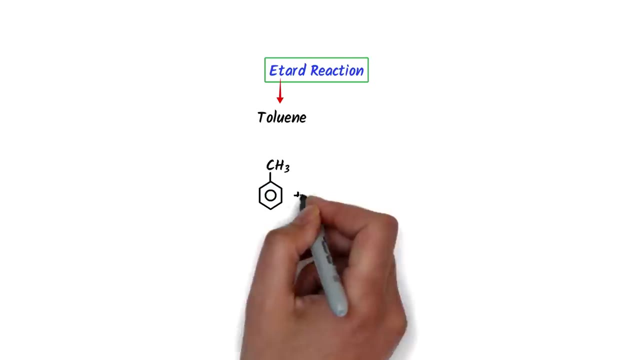 high. So this is the Stefan reduction reaction. Now let me teach you Etard reaction. Well, this TN Etard reaction reminds me toluene, So I write toluene, which is CH3 plus benzene ring. Secondly, this E reminds me Elon Musk. We know that he is crazy and clever. This 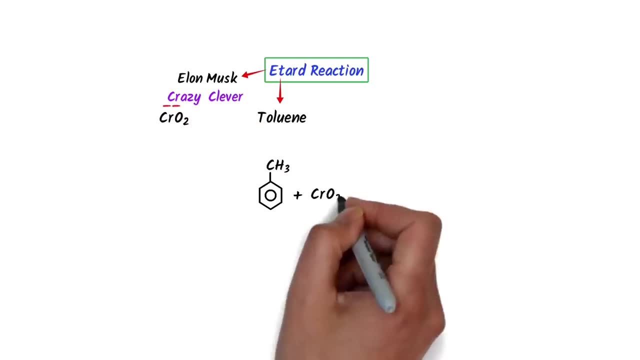 CR and crazy stands for chromium oxide and this CL and clever stands for chlorine. These are the reactants of this reaction. Now I replace these three by oxygen, I write CH plus benzene ring and I attach oxygen to it. I get benzaldehyde. So this is the Etard. 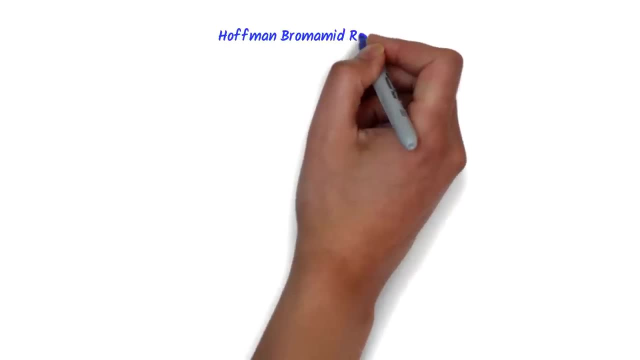 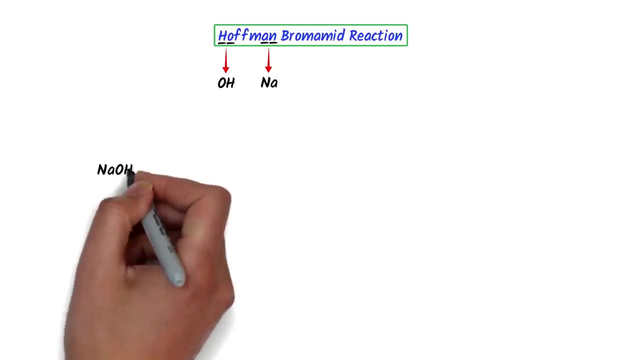 reaction. Now let me teach you Hoffman bromide reaction. Well, I select Na and OH and Hoffman. I write it as sodium hydroxide Plus. I select brom and bromamide, I write bromine. Thirdly, I select amide and bromamide. We know that amide. 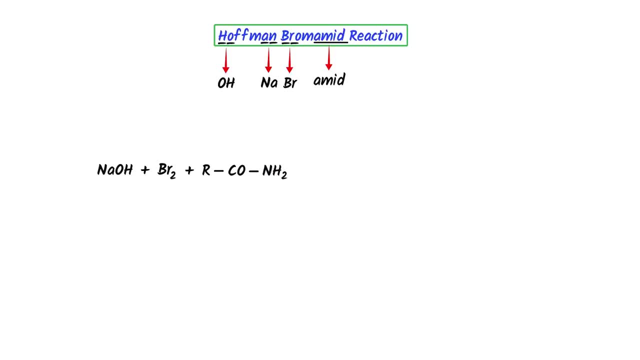 is R-CO-NH2.. So these are the reactants of this reaction. Now I break sodium and hydroxide. I break R-CO-NH2.. Sodium will attack on Br and CO. I get sodium bromide plus sodium carbonate. This R-NH2 will. 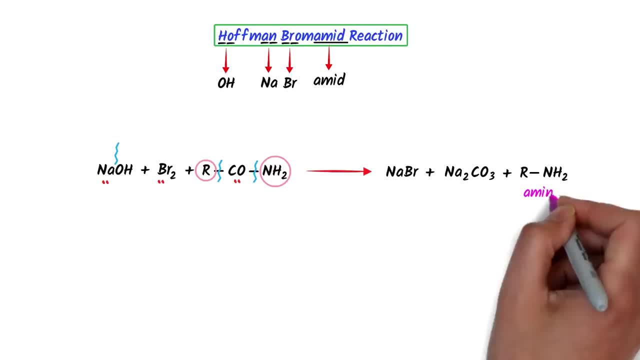 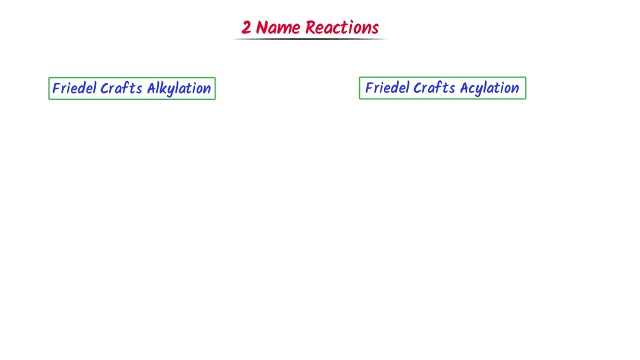 combine together to form amine. So this is the Hoffman bromamide reaction. Thus, note it down. Now let me teach you two more reactions like Friedel-Kraft's alkylation and Friedel-Kraft's acylation. Well, I always count the words of Krafts. 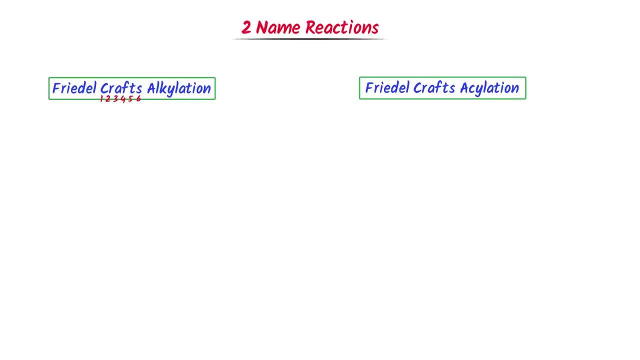 1,2,3,4,5,6.. These six letters reminds me the six carbon of benzene ring, So I write here benzene ring. Secondly, this A and L in alkylation reminds me AlCl3, aluminium chloride. 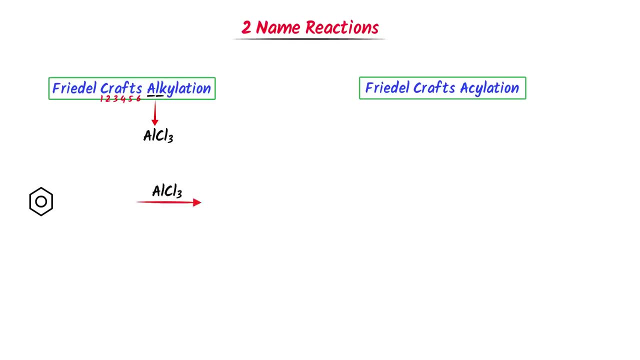 So I write here aluminium chloride. Thirdly, alkylation means alkyl halide like CH3Cl, So I write here CH3Cl3.. So I write here alkyl halide, So I write here CH3Cl3.. So these 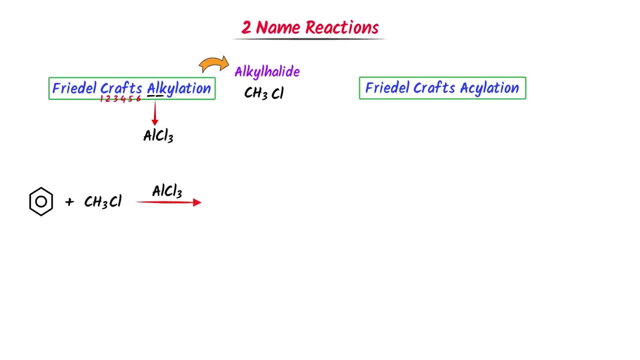 are the reaction. So let me teach you how to break sodium bromidane from Br and CO HCl. These are the reactants of this reaction. Thus I can easily guess its product. Now I cut Cl and I attach this CH3 to benzene ring. I get toluene. This is the Friedel-Crafts alkylation. 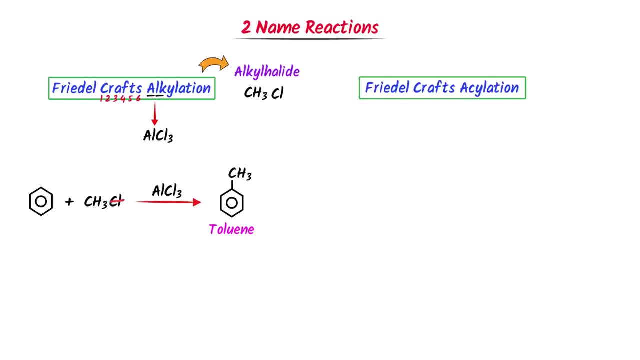 In case of Friedel-Crafts acylation, I take benzene and HCl3 and I write them here. Now. the word acylation means acyl halide like CH3COCl. I write here CH3COCl. We know that. 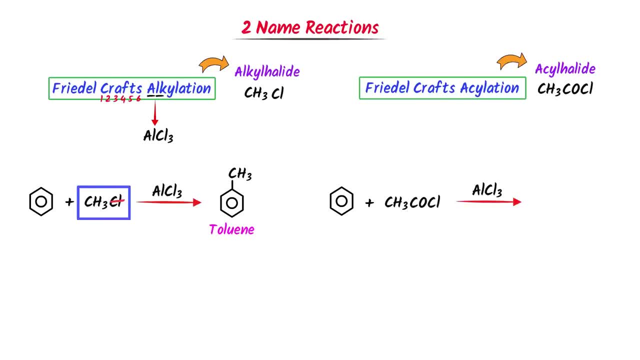 here we cut Cl. Similarly, I also cut here Cl. I take benzene and I write it here. Lastly, I go from back to right: CH3CO. I mean I write CO and then CL, I get acetophenone. This is the Friedel-Crafts acylation. So note it down, these two reactions. 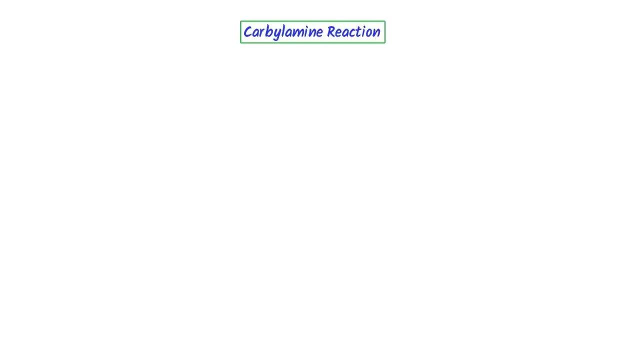 Now let me teach you carbyle amine reaction. Well, in carbyle amine, I select C and B. This C stands for chloroform. Its formula is CHCl. This B stands for base like sodium hydroxide. Secondly, I select amine, The formula of amine. 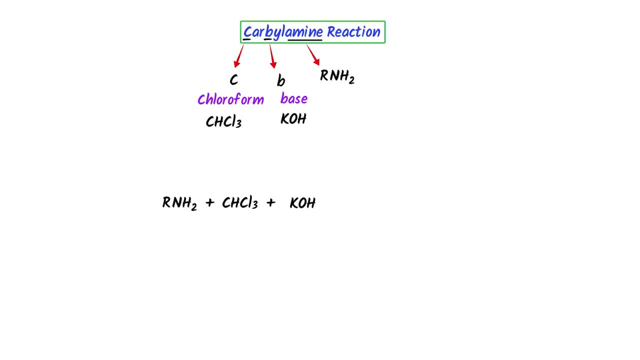 is CHCl. This B stands for base, like sodium hydroxide. Secondly, I select amine. The formula of amine is RnH2.. So these are the reactants of this reaction. Now, this will displace this H2. I get RnC. We call this compound as isocinide. Also, this K will attack on chlorine to form. 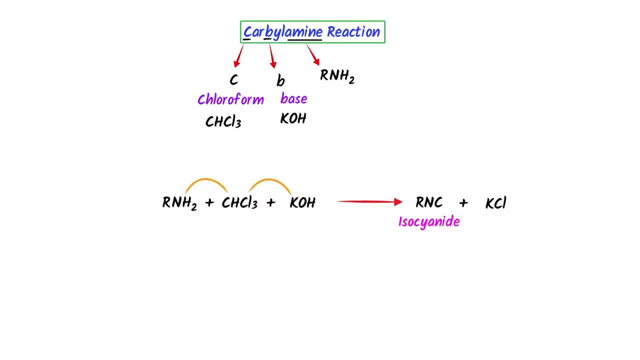 potassium chloride. Remember that this reaction is only possible in case of primary amine or 1 degree amine like CH3CH2NH2.. It is not possible in secondary and tertiary amine. Let me teach you HVZ reaction. Well, this H and HVZ always reminds me. alpha hydrogen is displaced. 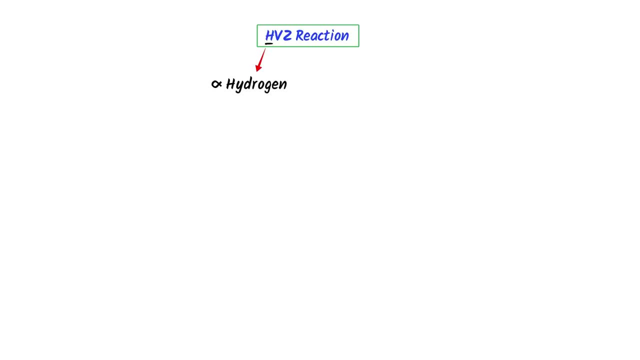 Now what is alpha hydrogen? I write carboxylic acid group like COOH. I attach one carbon and one alkyl to it. Now this adjacent carbon or second carbon after this carbon is called alpha carbon And the hydrogen attached to it is called alpha hydrogen. 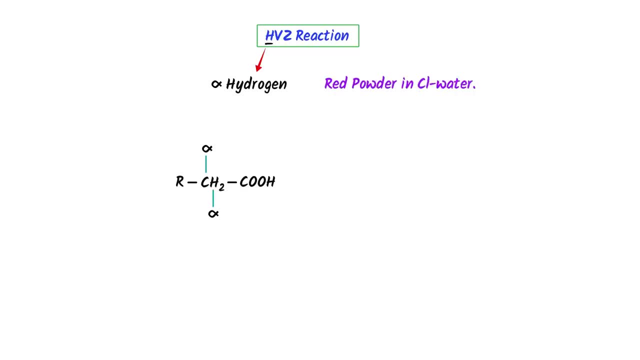 Secondly, I write a red powder and chlorine water. This red and P of powder stands for red phosphorus, Cl stands for chlorine gas and water is H2O. These are the reactants of this reaction. We already know that alpha hydrogen is displaced. 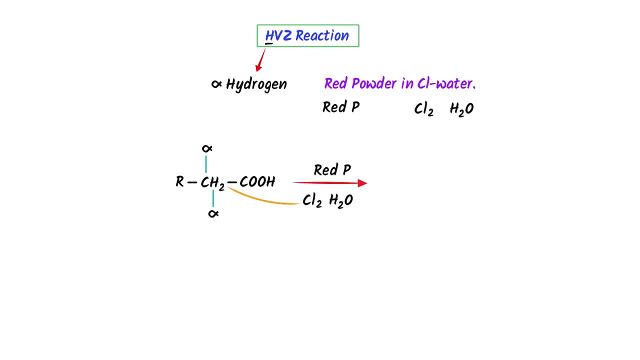 So this chlorine will displace one alpha hydrogen. I rewrite the compound. In case of one alpha hydrogen, I write chlorine to alpha carbon. Remember that this reaction is used for the halogenation of carboxylic acid. Now let me teach you two more reactions. 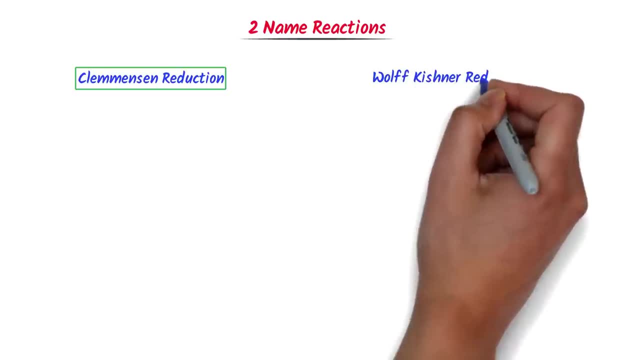 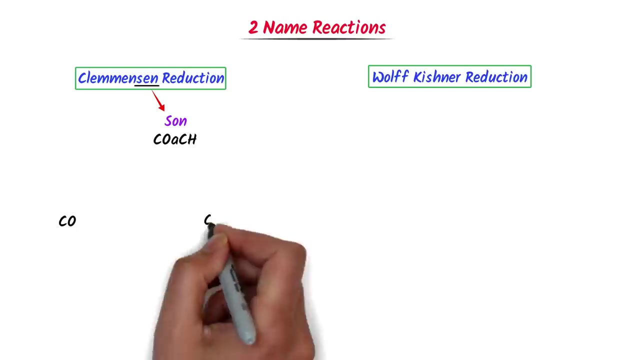 Clementson reduction reaction and Wolf-Kishner reduction reaction. Now listen carefully. In the Clementson there is a word: sun. We know that every sun needs a coach. Remember that I write here CO and I write there CH. Similarly, 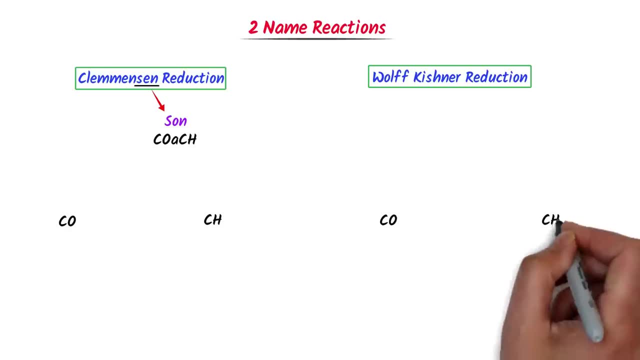 I write here CO and I write there CH. This CO is the reactant and this CH is the product. Also, this CO is the reactant and this CH is the product. Now, what about the other reactants of Clementson reaction? Well, this CL reminds me HCL. 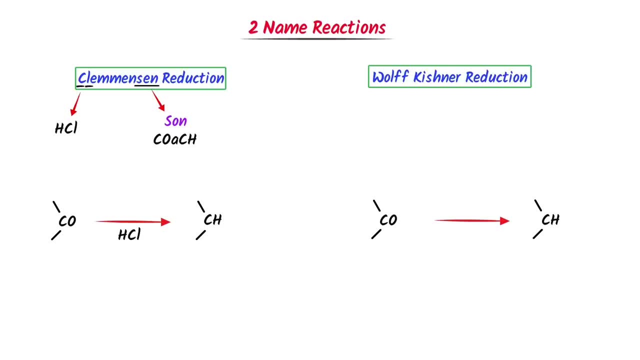 So I write here HCL. Secondly, this MM reminds me a zigzag line. Here this Z stands for Zinc and G stands for HG, So I write here Zinc and HG. This is the complete Clementson reaction. Now what about the other reactants of Wolf-Kishner reduction reaction? 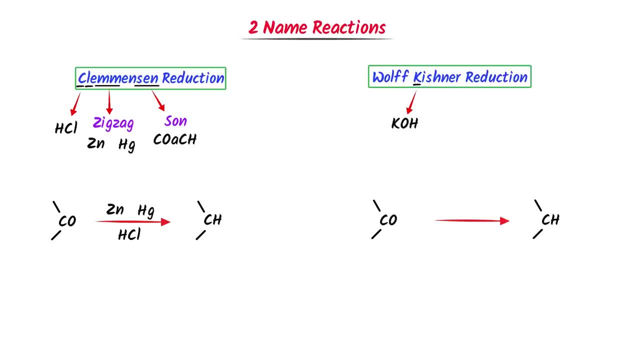 Well, this KN-Kishner reminds me Potassium Hydroxide. I write here Potassium Hydroxide. Secondly, I select this N and H. It reminds me NH2NH2.. So I write here NH2NH2.. This is the complete Wolf-Kishner reduction reaction.